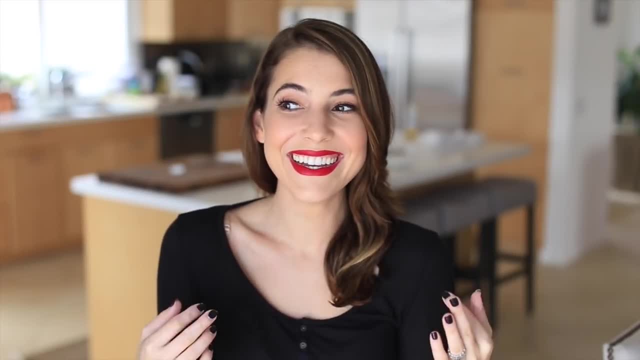 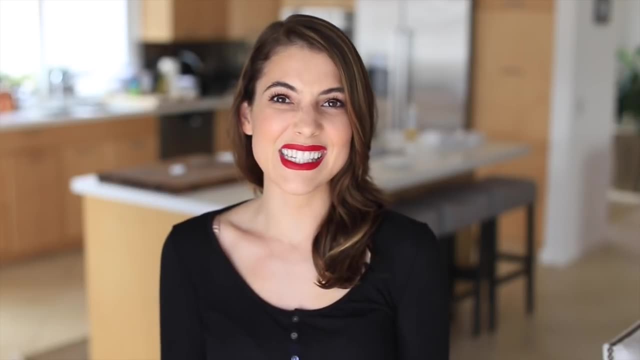 a lot when I was pregnant. I did a ton of pinning when I was pregnant, hoping that I would definitely get around to it at some point. So now that he's a toddler, I'm definitely trying out some of the ideas, like the fun little games and do it yourself crafts, and 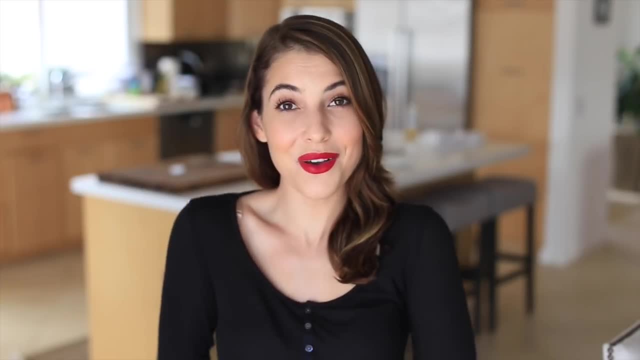 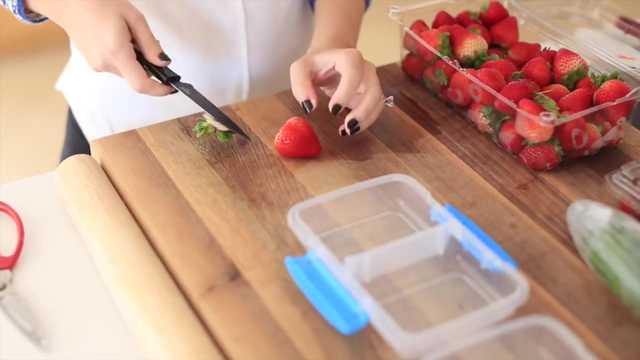 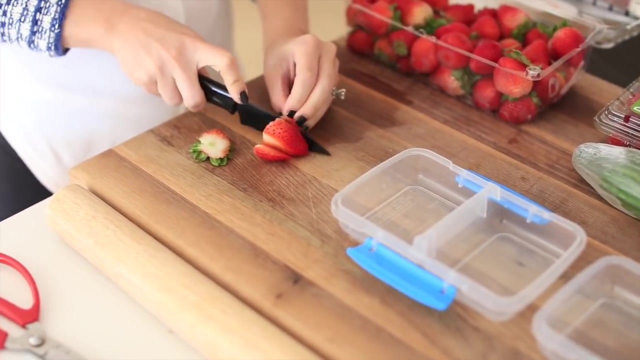 food and snacks and things like that. So hopefully you guys enjoyed this video and, yeah, we'll just jump right in. So snacks are great and all, and I definitely love to treat Oliver to crackers and various bars and things like that, But I always try to maintain fruits and vegetables as much. 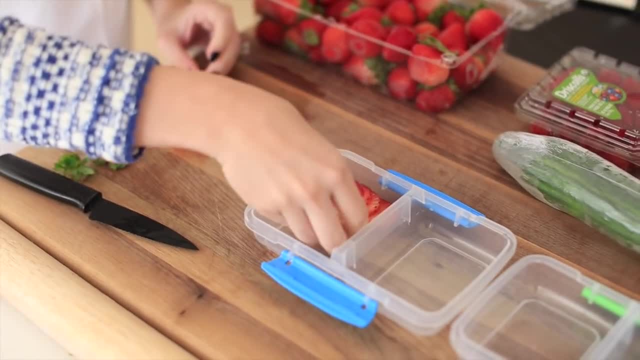 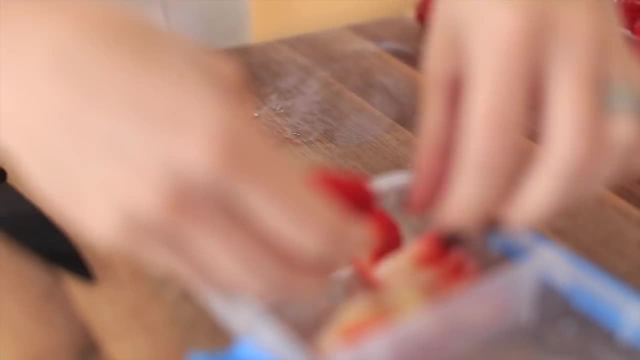 as I can. in his diet He really, really loves berries. He does love carrots and cucumbers, So I make these little snack pods. You can add anything you want to these snack pods. It could be cubes of cheese and pretzels. But I try to do really really healthy options. 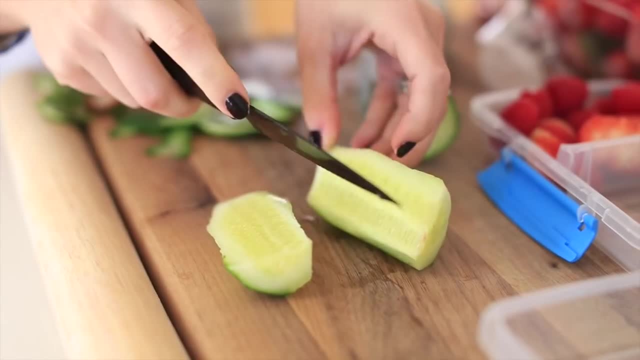 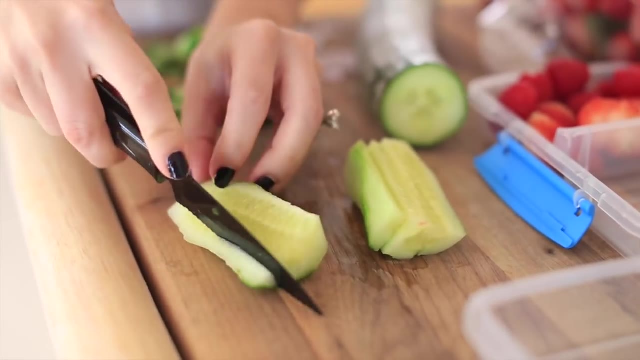 But since I know my son will just devour berries, I will have a side for berries and then cucumber and some carrots. I will put them in these little snack pods. If he asks me for a snack- which he'll usually come over and let me know like: hey, mom, I want a snack- I'll ask him. 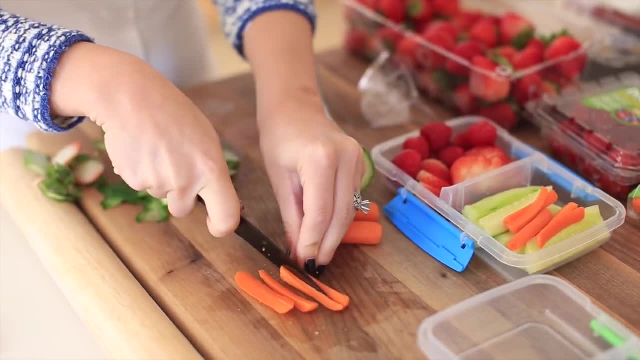 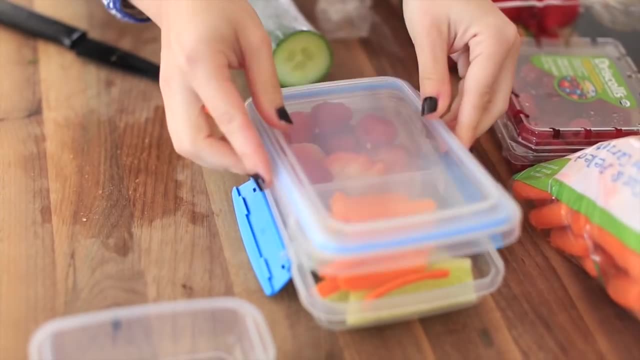 if he wants a snack, I will have a few of these ready to go. They're only good once you cut the veggies and fruit for about maybe three days, So I will premake these and offer it to him if he asks me for a snack. if he doesn't finish it all, I'll put it. 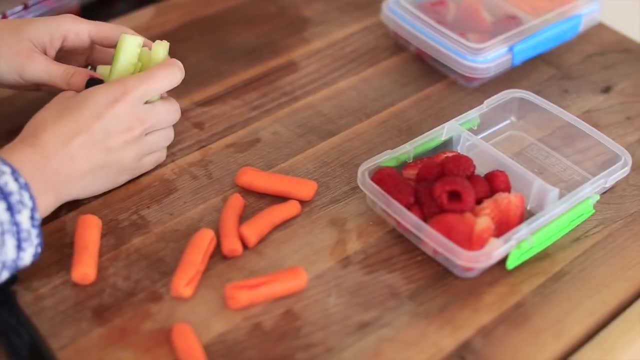 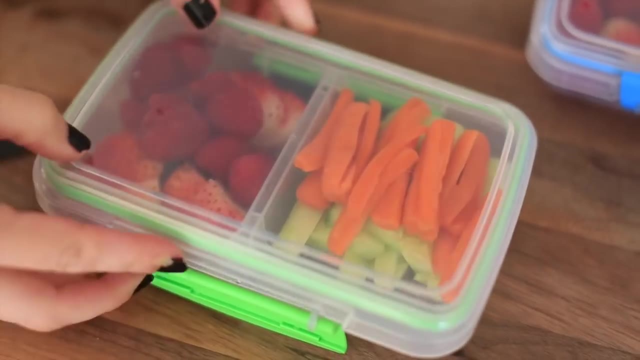 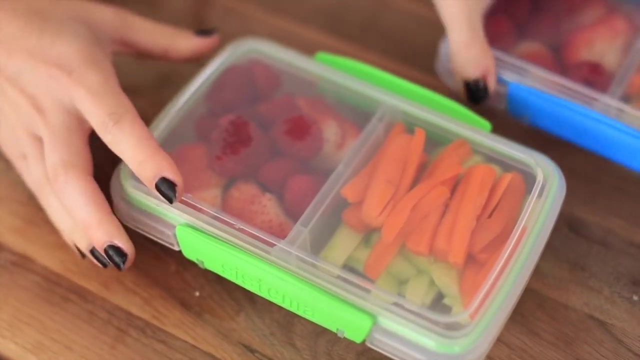 back in the refrigerator. but I just like to have these healthy options ready to go on hand and just I know with the cucumber it's already cut, it's just the perfect size for him to eat. snack pods are definitely a quick and easy way to feed your toddler something healthy, and even older kids you could definitely put. 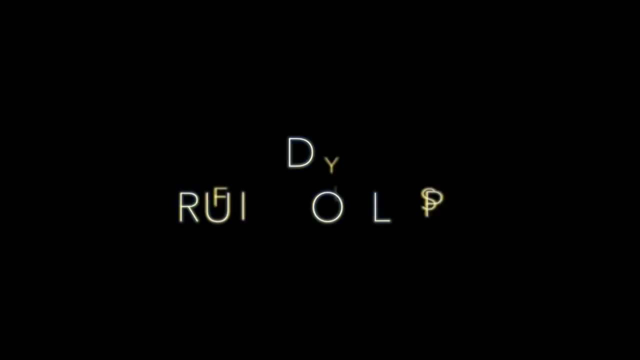 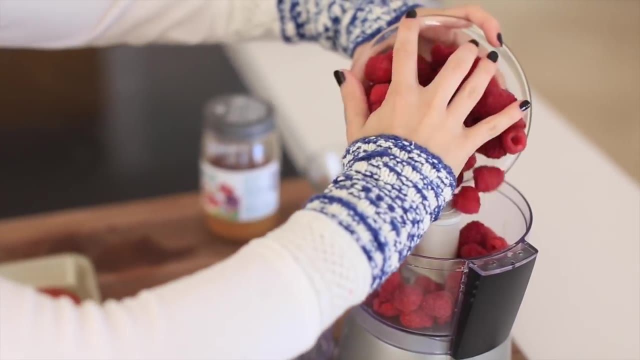 this in their lunch boxes. next up, we have fruit roll-ups, which I've been seeing all over Pinterest and just dying to make for Oliver because I remember I used to love fruit roll-ups. so I will have the full ingredient list, of course, in the description, but 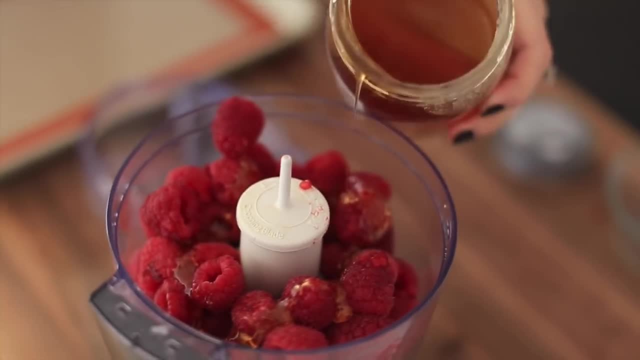 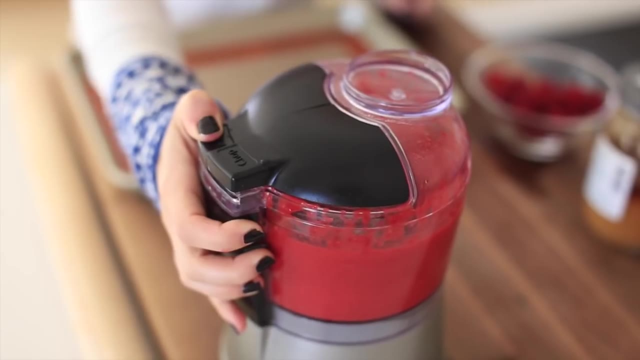 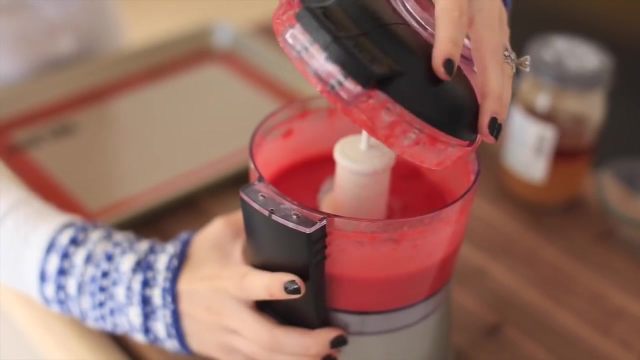 basically it's just honey which I have, this, this honey that I get from sprouts and some organic berries, and I put that all in my food processor and just process that away and then I just you're just gonna pour it on a silpat and you're gonna put some on a plate here and I'm gonna put the rest of this fruit roll-ups in. 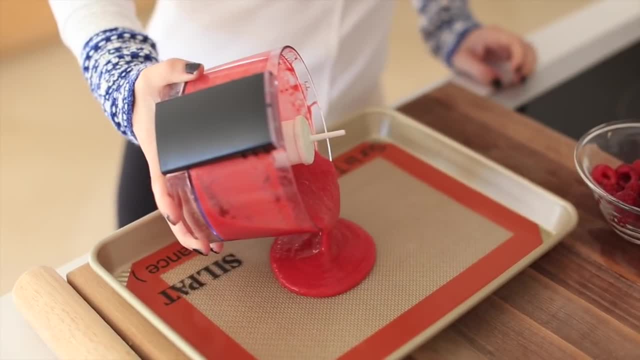 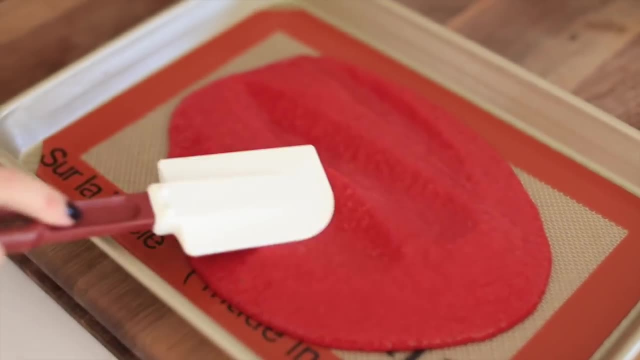 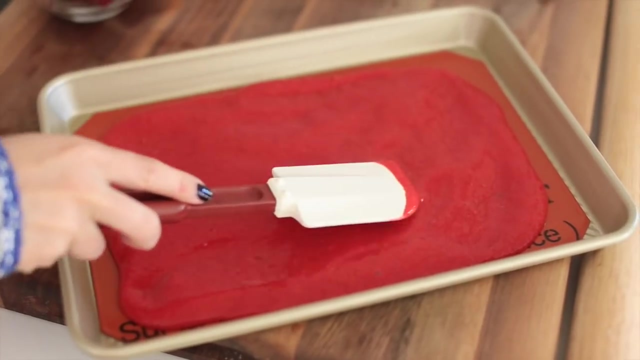 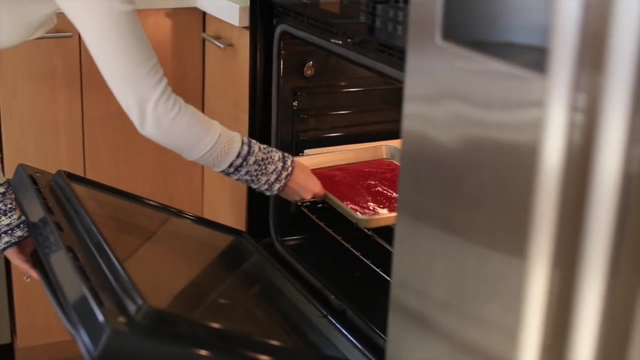 gonna actually cook it and you're gonna bake it, for I think it's about six hours. it's definitely a long time, so keep in mind that it's basically just dehydrating it, So after what seems like an eternity in the oven, 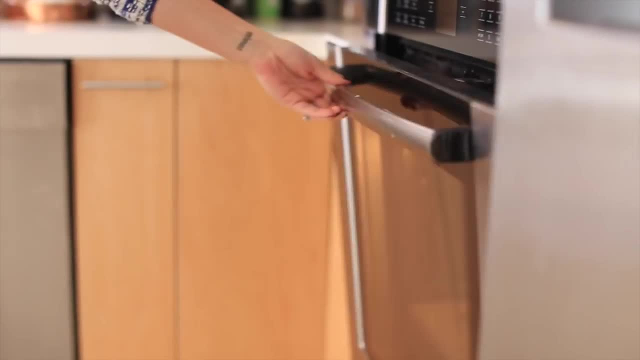 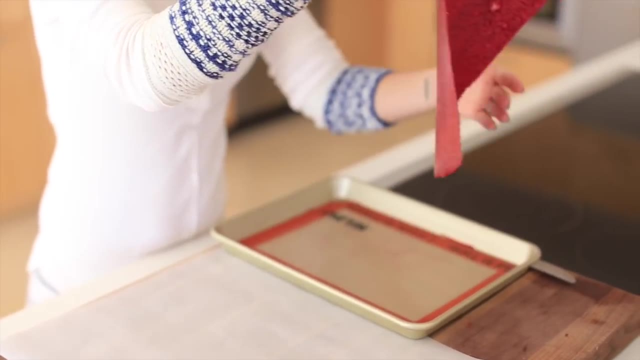 you're gonna take it out and it's actually dehydrated at that point, which is fabulous, because you can just pull it right off the baking sheet, and then you're gonna put it onto some parchment paper and then you're just gonna roll it. 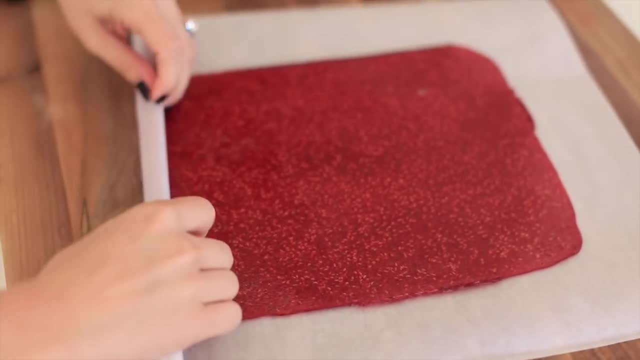 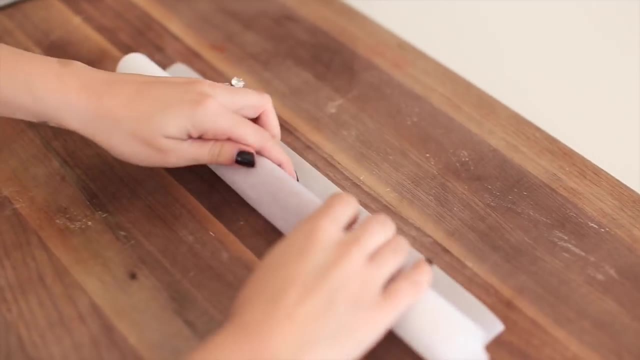 just like you do with the traditional fruit roll-ups, and then I like to cut it to make them smaller portions. There's another option that you can choose to do, and that's to strain the seeds. Looking back, that might be something I do. 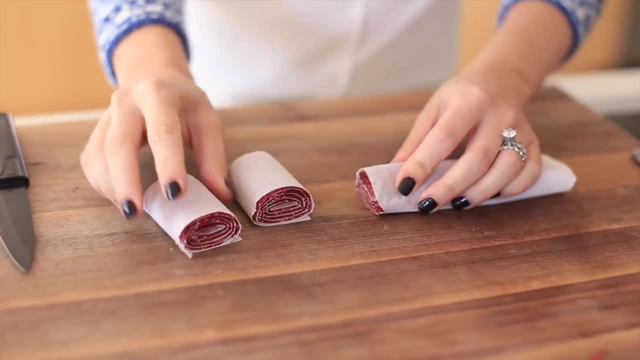 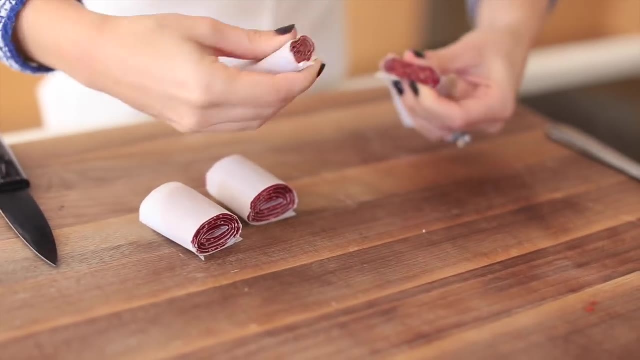 if I ever make this again in the future, which I do think I will do, because my son really really liked this a lot. He's a big fan of berries on their own and this is just berries with a little honey. You can add more or less to your taste. 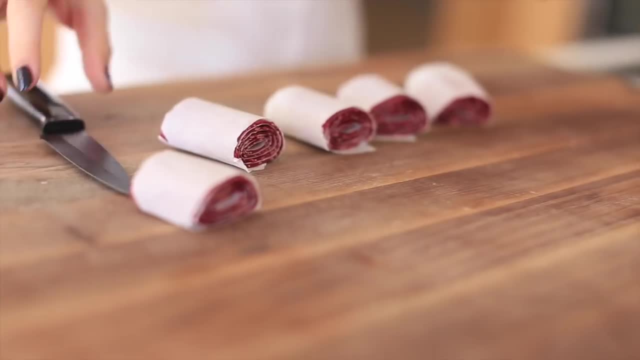 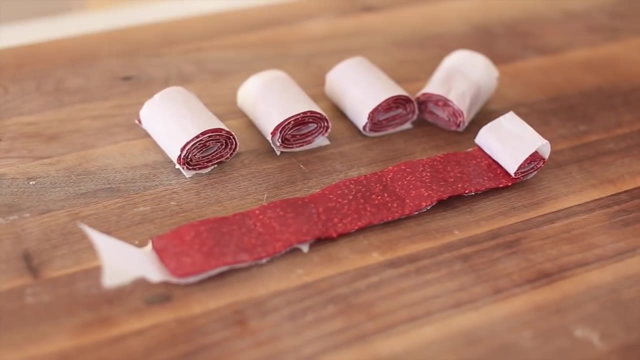 but these were pretty tart so they weren't super-duper sweet and he still really liked them as a special treat or snack and especially if you're potty training or you're around that age, this is a great snack or treat if they've used the potty. 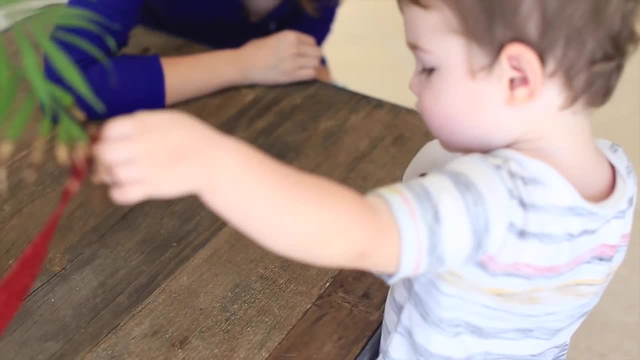 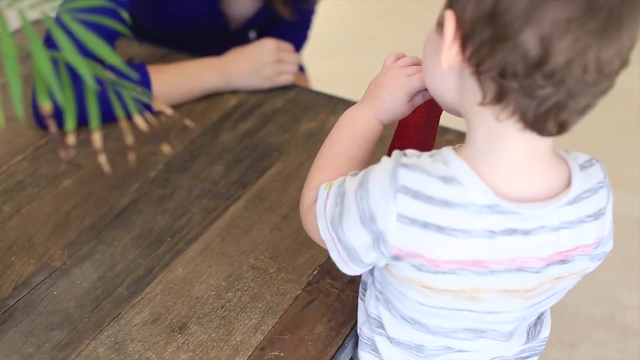 or it's good reinforcement. So the bottom line is that I'm a big fan of these and I definitely divided them. I didn't give them all to him at once, because he went crazy and wanted more and more and more, but it just I don't know. 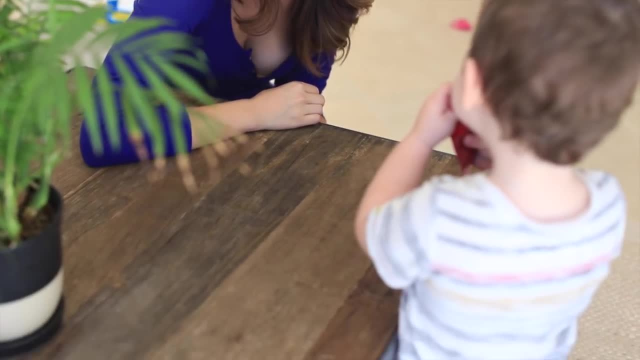 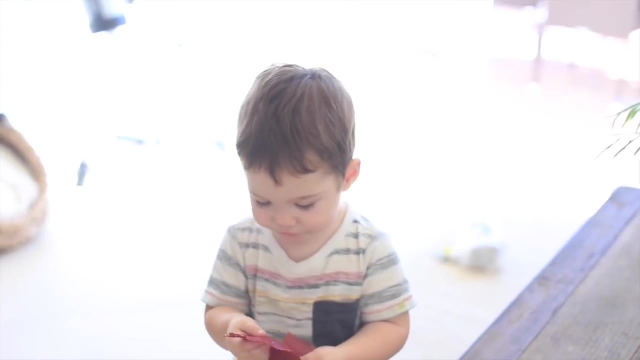 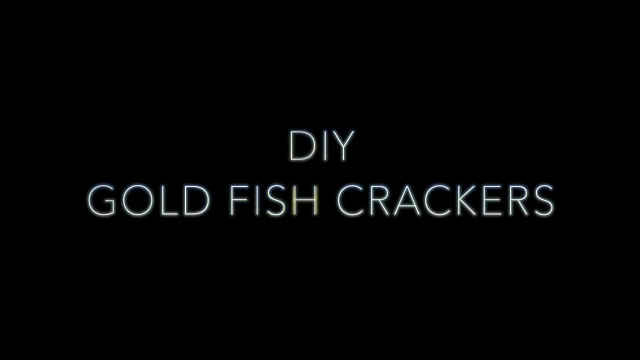 it brought me back to my childhood and how much I loved Fruit Roll-Ups and I was glad that he liked them and just to know what actually went inside of them. But yeah, big hit. Next we are making homemade goldfish. 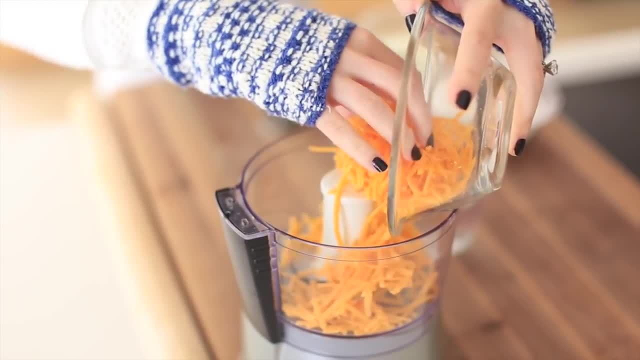 which is another one that I saw on the internet and I was like, oh my gosh, this is so good. I saw it on Pinterest and just had to try, and I was so amazed by this recipe. I just loved it. 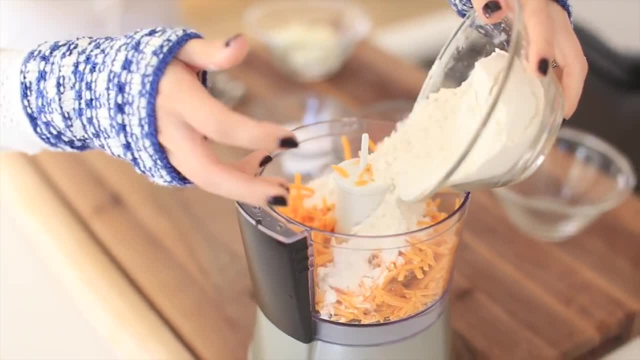 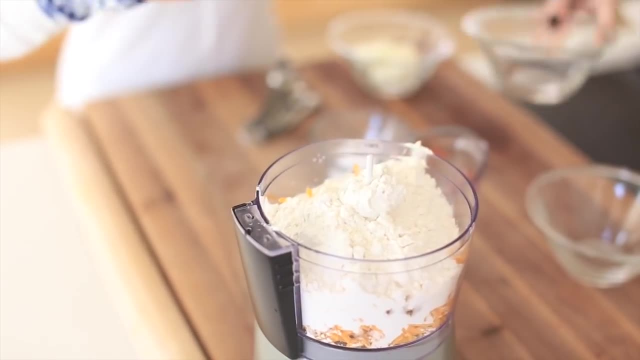 So again, full recipe will be in the description, but I'm just adding cheddar cheese and some flour. Now, of course, if there's a type of flour that you like to use for your children, you can certainly use that and make it even more of a healthy option. 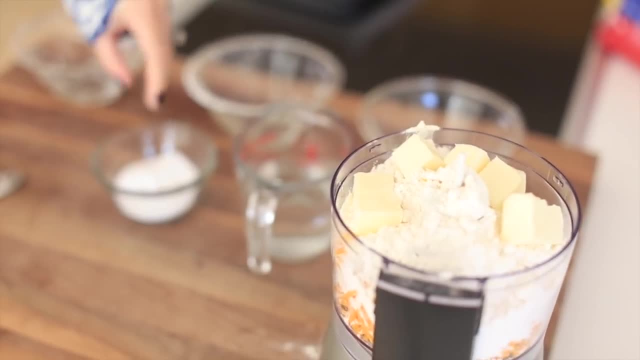 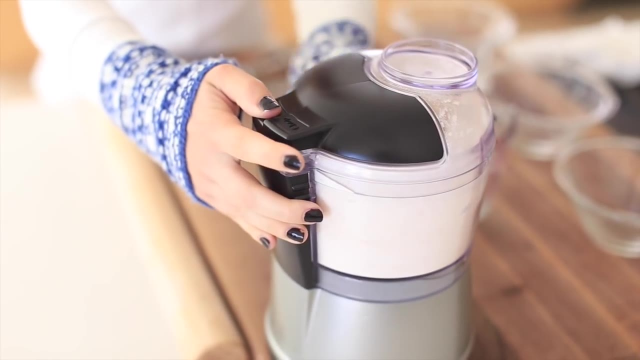 I just like that these are made from home and obviously just some butter and a little bit of salt, And then again I'm gonna put it in the food processor and just go ahead and just process it until you really start to see the color come out- the cheese. 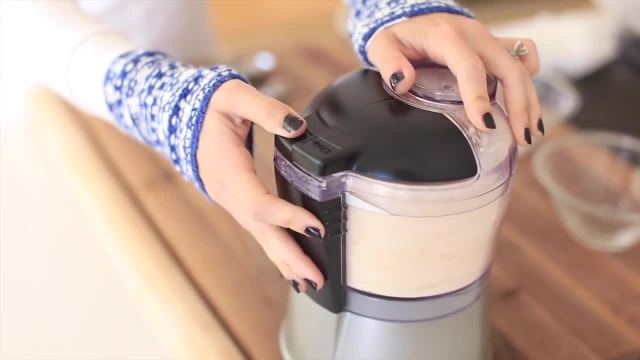 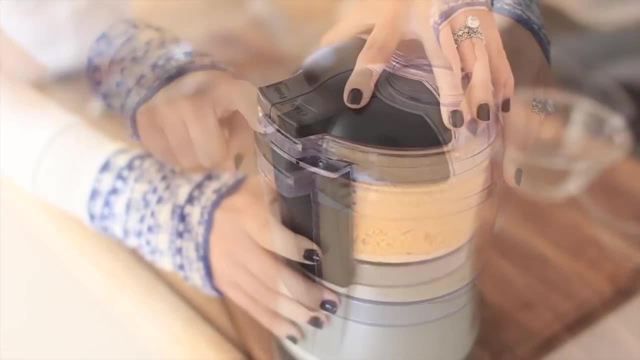 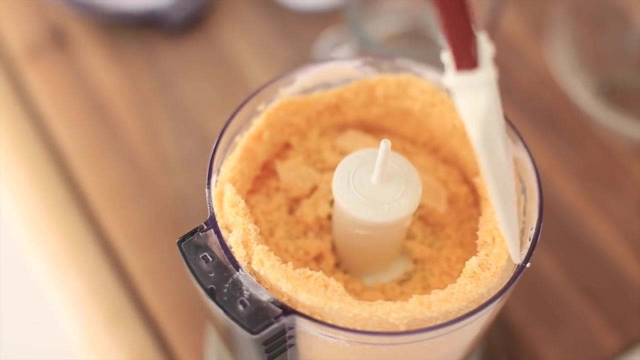 and you'll see that the cheese will really start to make its appearance as it becomes more and more orange. So I'm gonna go ahead and remove the top of the food processor, I'm gonna take a spatula and just kind of push everything down in the middle. 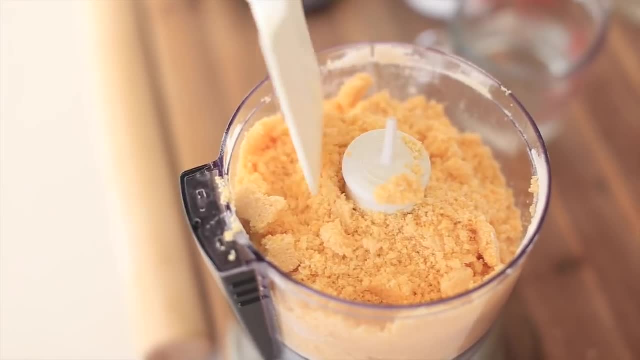 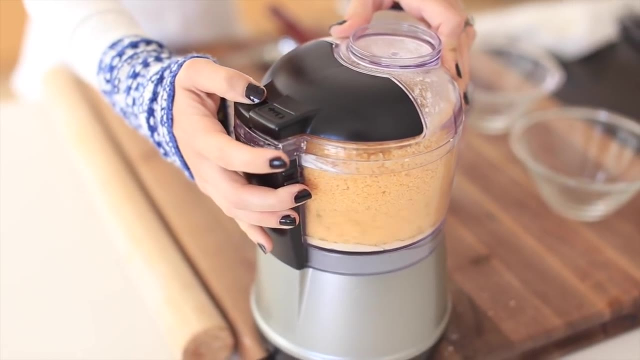 and go ahead and just process it one more time through to just make sure it's really really smooth. You just want like a sandy texture And then to remove the top again and slowly add a little bit of water. I believe it's a tablespoon at a time. 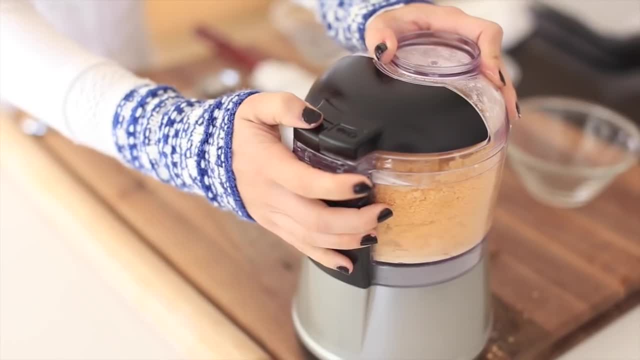 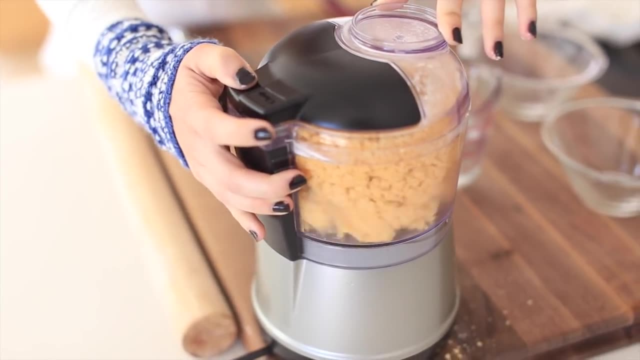 and we're gonna do two. So I'm gonna add a little bit. I'm going to run it through the food processor, take off the top, add a little bit again, run it through the food processor and then we're gonna have the dough. 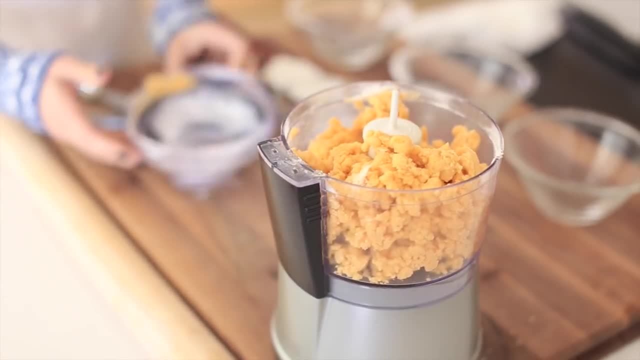 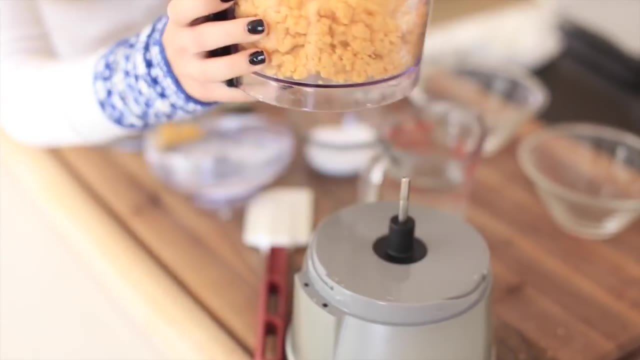 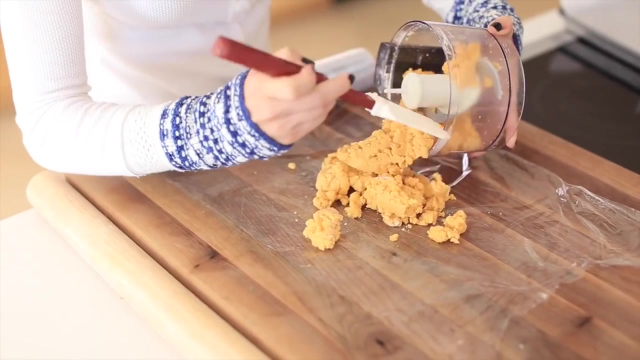 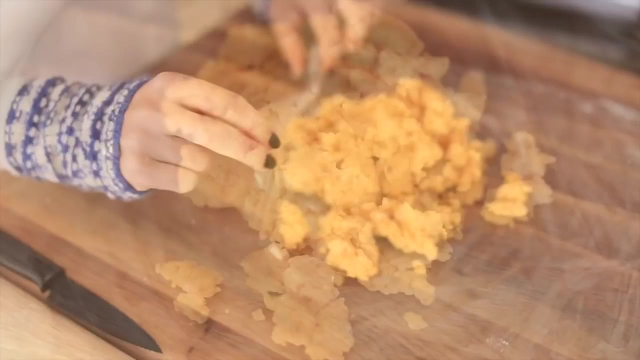 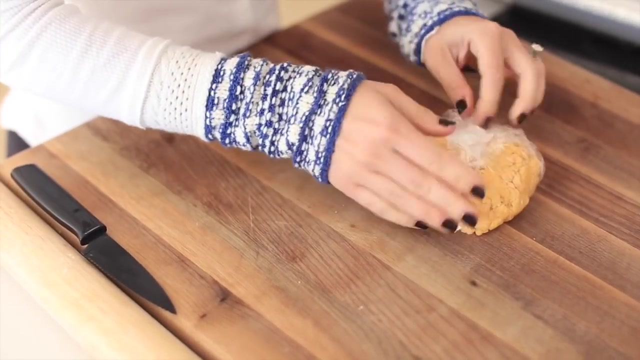 that we need to make our goldfish With a spatula. I'm gonna take the dough out of the food processor and onto some plastic wrap because it needs to chill in the refrigerator for about 30 minutes. While the dough chills in the refrigerator: 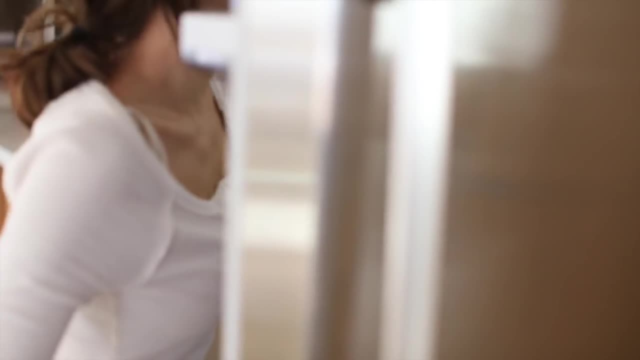 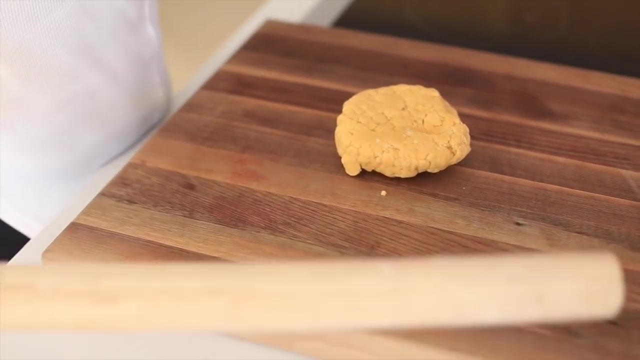 be sure to set your oven to 350 degrees, which is the temperature that it needs to be at when you cook. After the dough has chilled for 30 minutes, you're going to roll the dough out, And then these taste very, very similar to Cheez-Its. 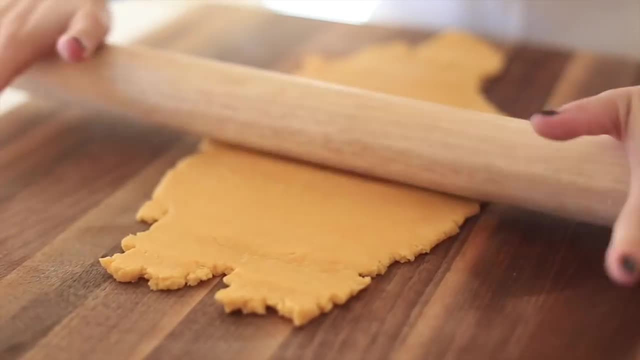 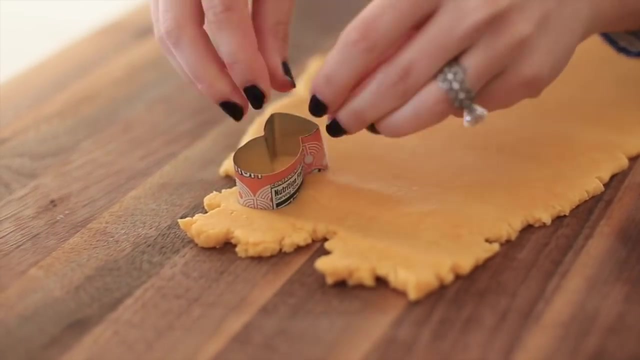 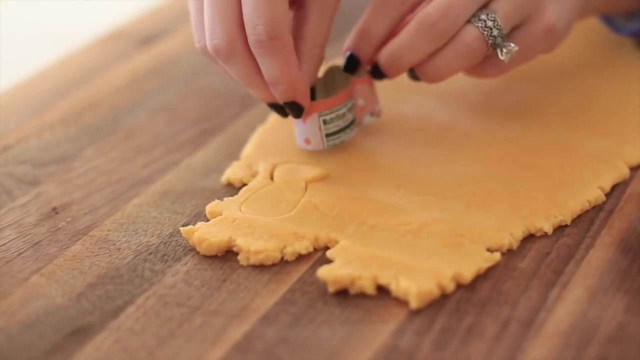 and also goldfish, So you can make squares if you want. I actually made a little fish out of a Perrier can and used that to create the little fish Now, obviously it's bigger and thicker than a traditional goldfish, but it tasted just like it. 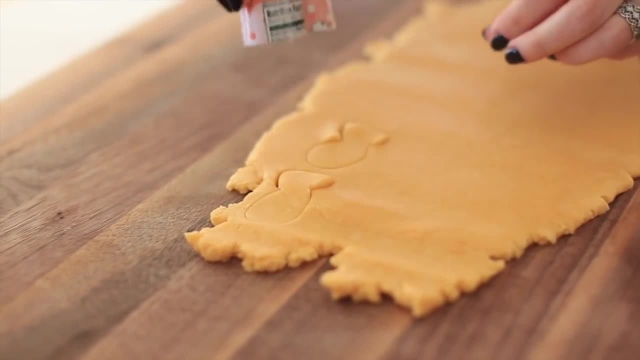 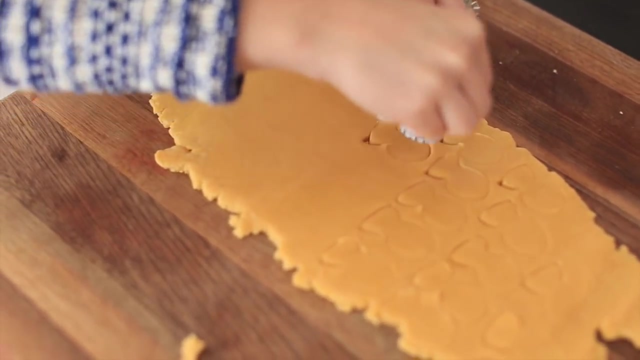 And I have to say I even got my chef husband to approve. he was eating them and he said, wow, those taste really, really good. They tasted just like Cheez-Its and goldfish. We were so blown away So I just created a bunch of little cutouts. 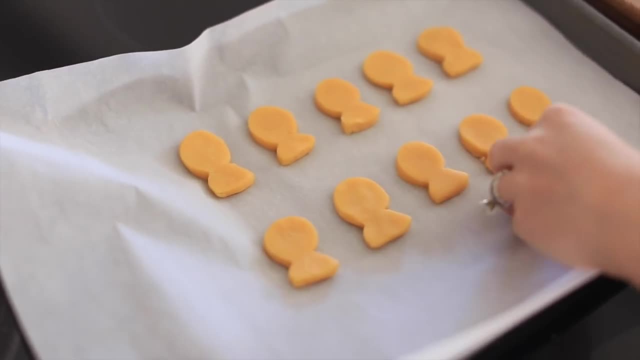 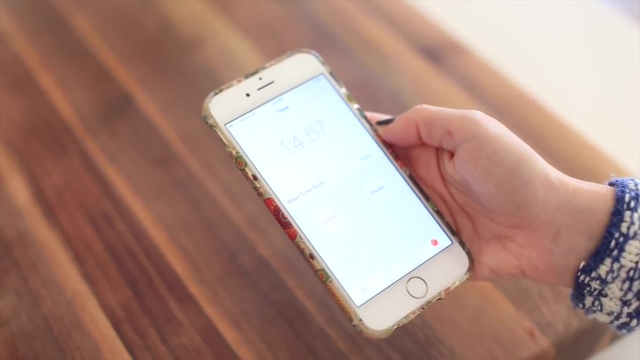 and put it onto a baking sheet and I'm gonna bake it for about 15 minutes, So it doesn't take very long at all. I left it in for about 17 minutes because I felt like at 15 minutes it needed a little bit longer. 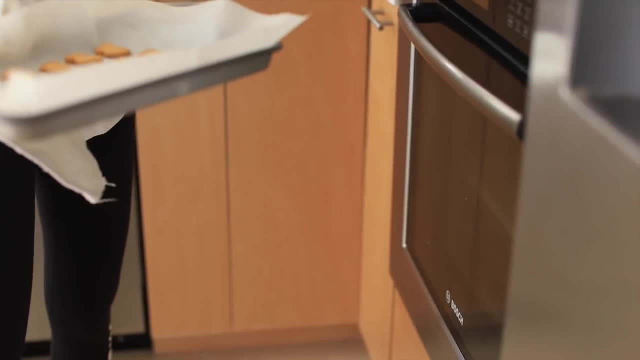 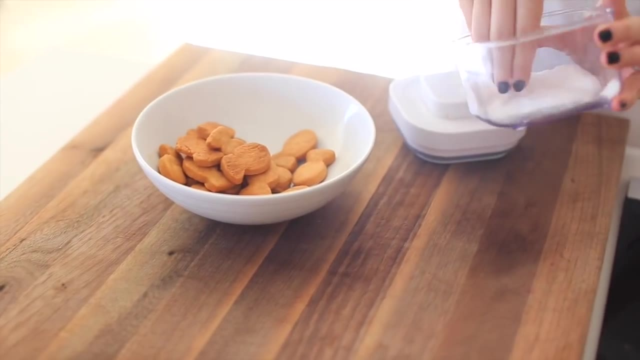 So I would say 16 minutes is probably the perfect amount to bake, depending on the temperature of your oven and how your oven works, exactly, But about between 15 and 17 minutes. I added a little bit of salt on top and this is obviously a special treat. 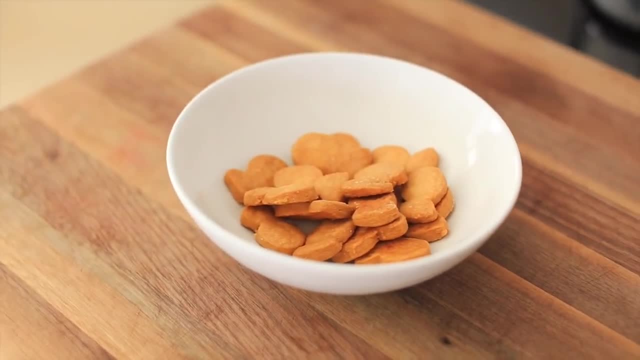 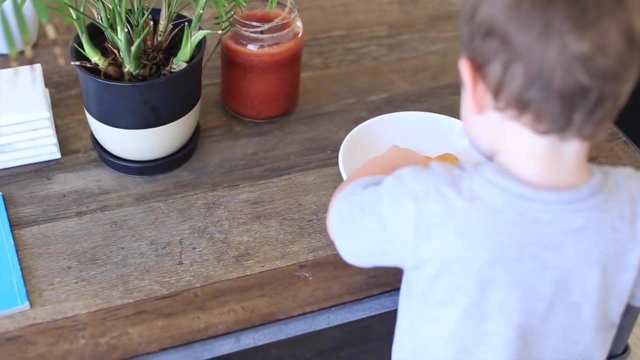 that looked like a lot of salt, but it really wasn't that much. I promise This was a special treat for Oliver and I loved them. He loved them, Byron loved them. They were definitely a hit for the family, So I would definitely try these out. 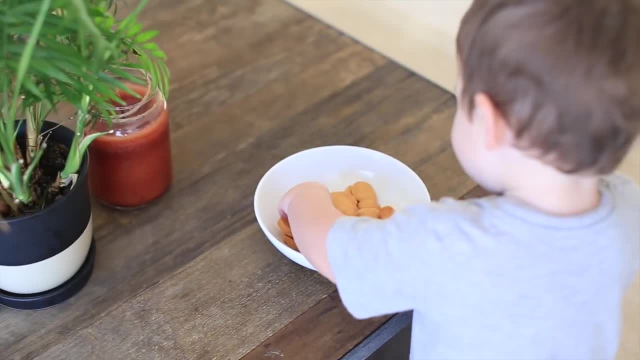 It just it feels good to know that you made, even if it's kind of I don't know 10 or 15 minutes. You made a guilty pleasure snack, Like you made it at your own home and you know everything that went in there. 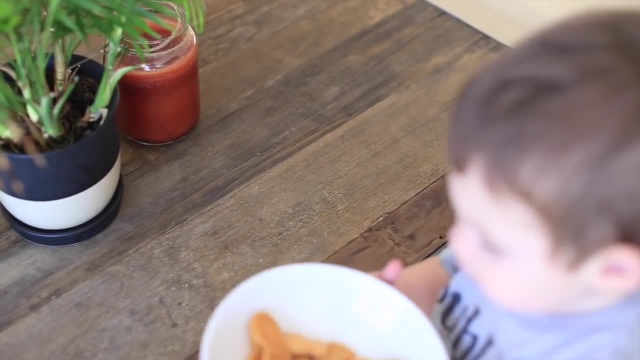 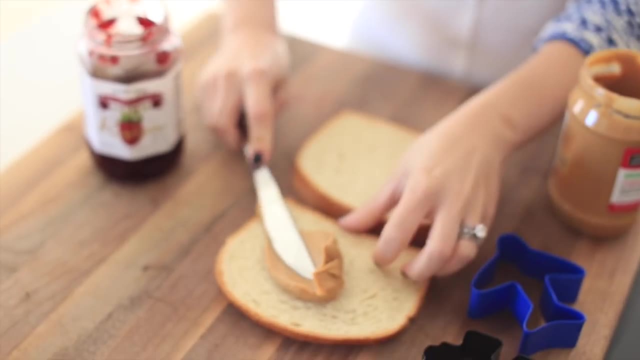 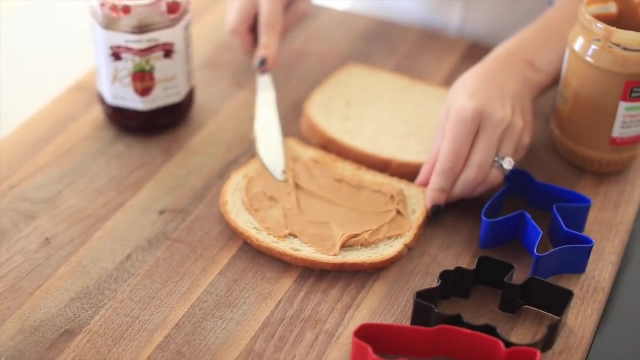 So yeah, those were a hit. So I don't know about your house, but in my house we definitely love peanut butter and jelly sandwiches. I mean, come on, Doesn't every toddler love a peanut butter and jelly sandwich? So when my son goes to grandma's house, 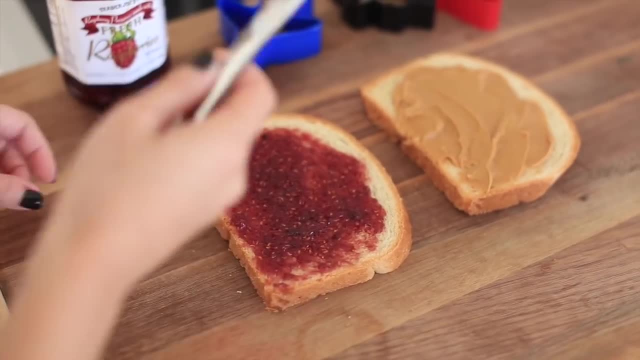 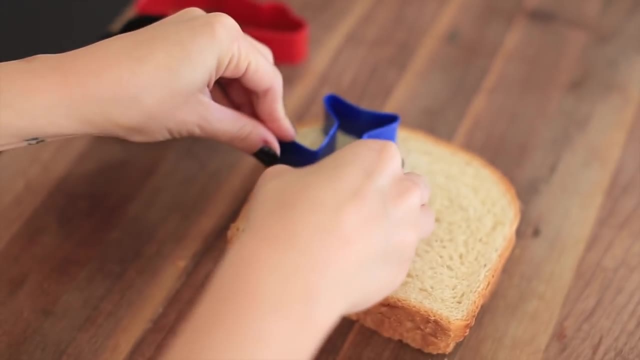 she always has the Uncrustables And she feeds them to him because he loves them, So I'm like I could make that. Obviously I don't like to waste, So I do eat the edges because I just feel bad throwing it away. 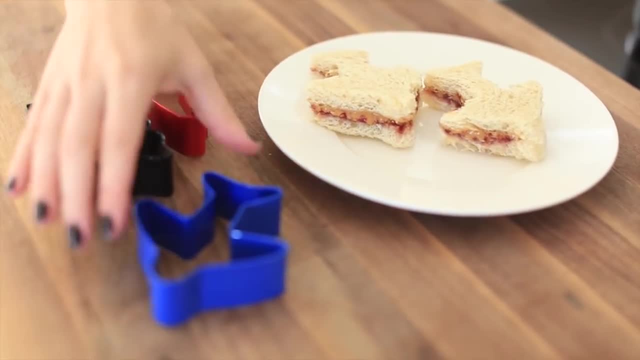 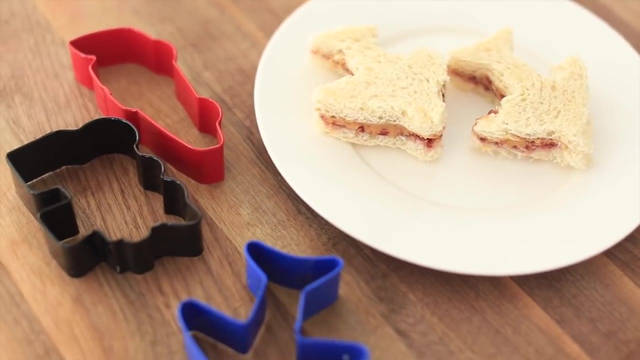 But I do make these little airplane shape kind of like Uncrustable peanut butter and jelly sandwiches for Oliver And he just loves them. I mean they're the perfect size, You can pre-make them. He always plays with them because he thinks they're actually like airplanes. 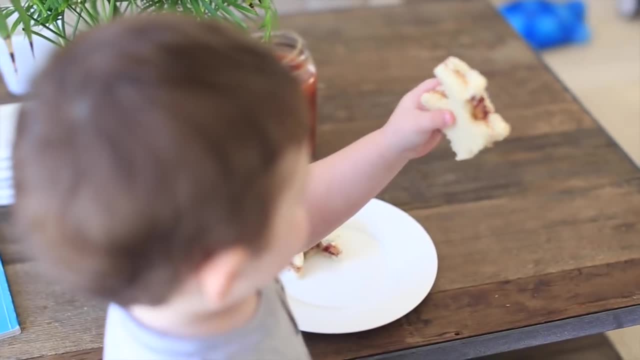 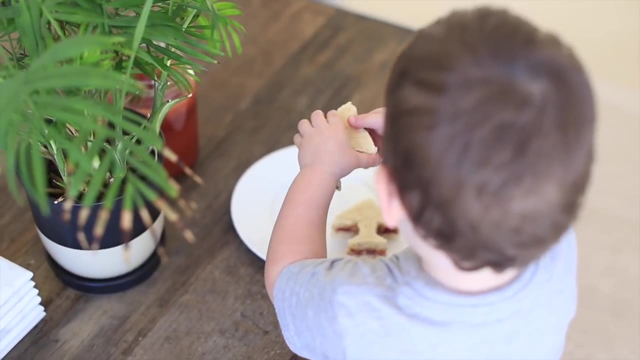 So he'll like make the noise, Like right now he's making the noise He's going. But it's just a fun, really easy, very, very easy. I think most moms kind of do this for their kids. Peanut butter and jelly sandwich are definitely a hit. 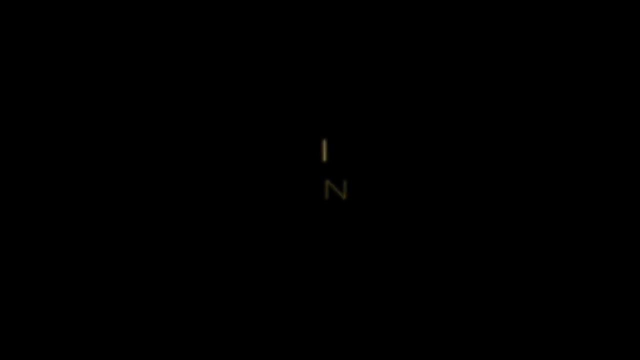 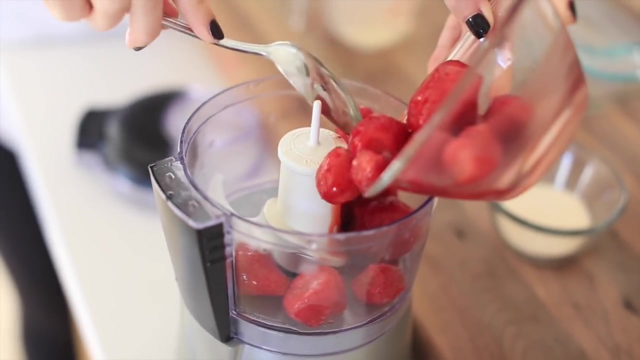 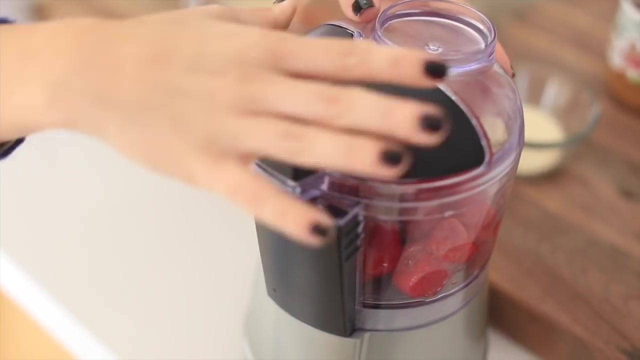 So I get those. at Target You can get those cutouts. And then, finally, we have fruit snacks, which, again fruit snacks- are another super yummy treat for kids. But it's good to know that you're making them at home and you're kind of controlling the ingredients. 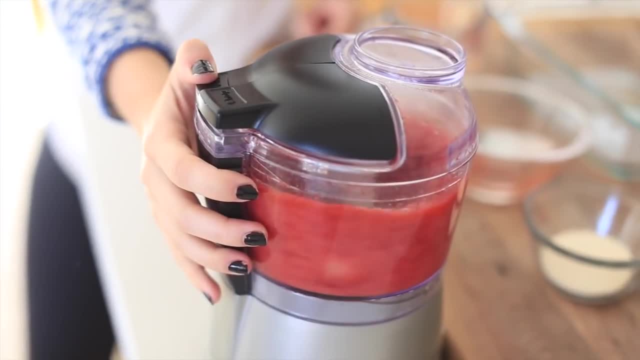 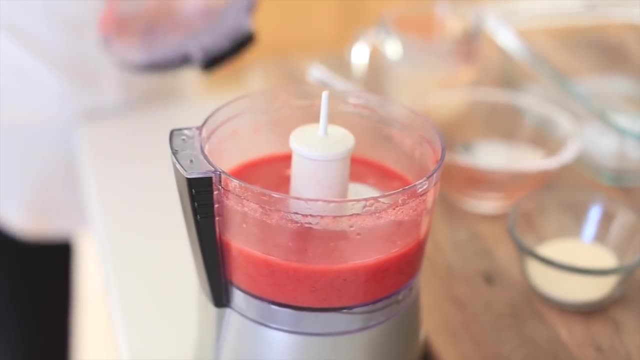 that go in there. So I'm starting again with the food processor. I have frozen berries that I've just kind of been sitting out for a little bit, So they're not super, super frozen. So I have the berries and I went ahead and processed those. 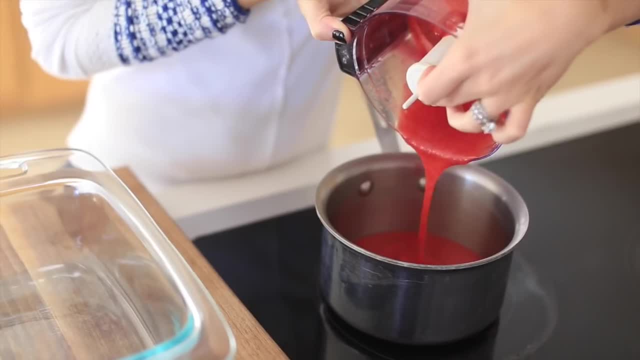 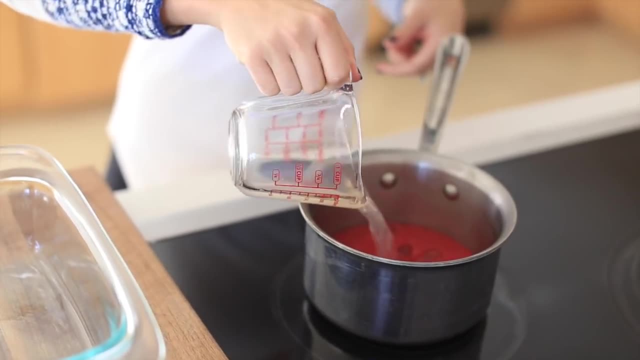 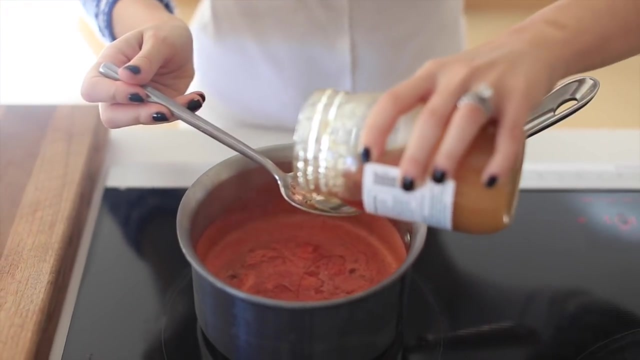 I'm going to put those into a pan, a stove top pan, and I'm going to cook it on medium to low heat. I'm adding some lemon juice and a little bit of honey. So in the sauce pan you're going to heat the strawberries. 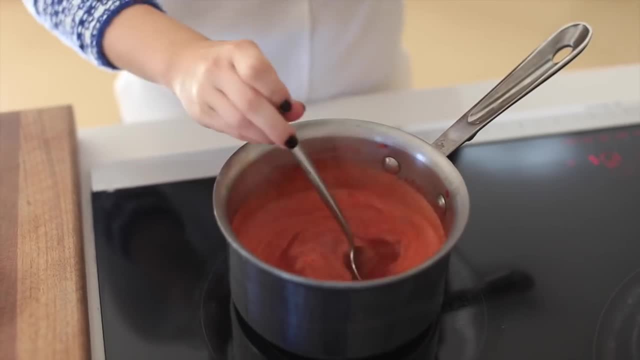 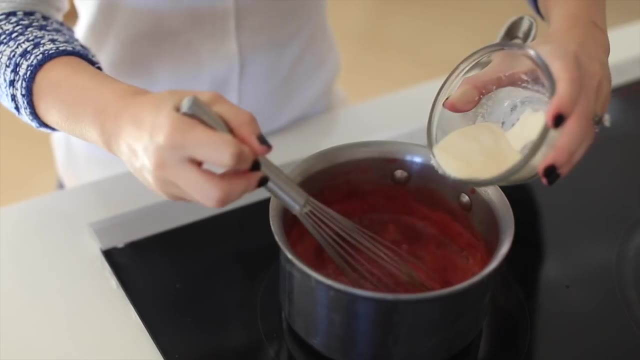 and the lemon juice and honey, And then you're going to slow. once that gets hot, you're going to slowly add some gelatin, Just slowly add a little bit at a time and whisk it in there. And the key is to really add a little bit at a time. 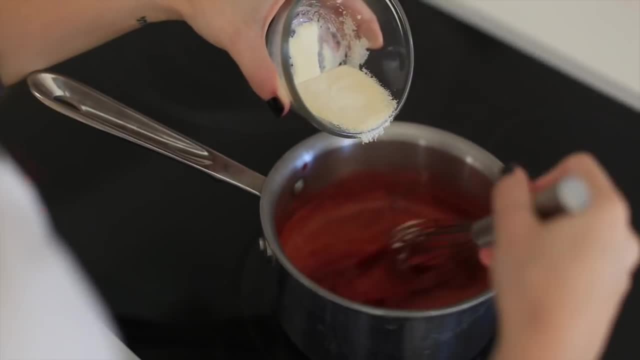 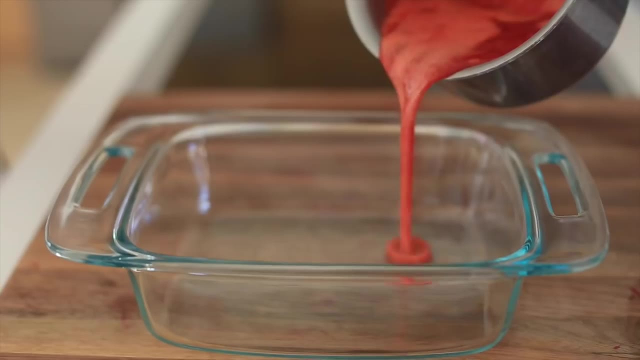 and make sure it is thoroughly absorbed so that you don't get lots and lots of clumps. So I'm going to go ahead and do that: You're going to let it reduce a little bit and then you're going to put it in a bowl. 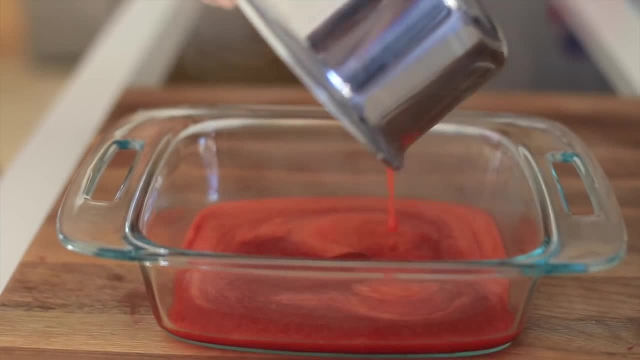 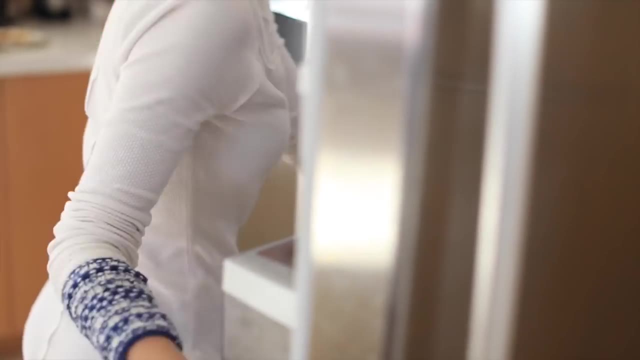 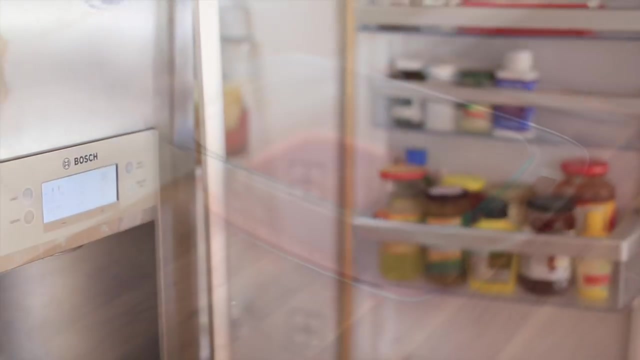 Put it in a pan and then you're just going to stick it in the refrigerator and let it refrigerate for about eight hours or overnight. So essentially these are basically like jello, but it was reduced a little bit more, so it's even chewier, like a fruit snack. 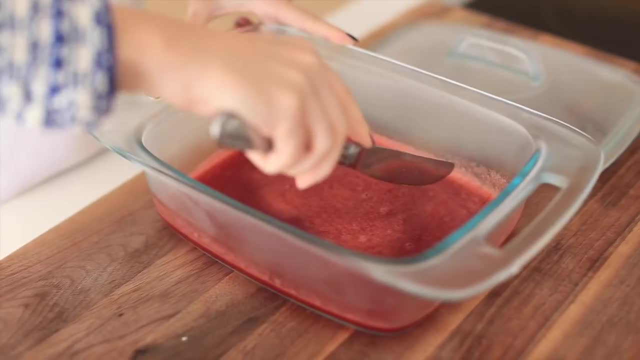 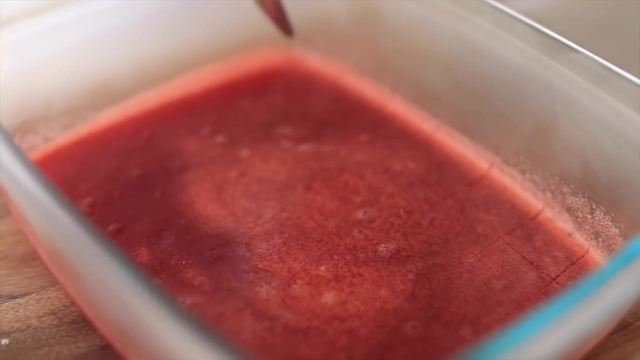 It's similar to a fruit snack, but it resembles jello a little bit more for me, And I left it out and it was a little warm and it kind of melted. I cut them into squares, but you could cut different shapes out. 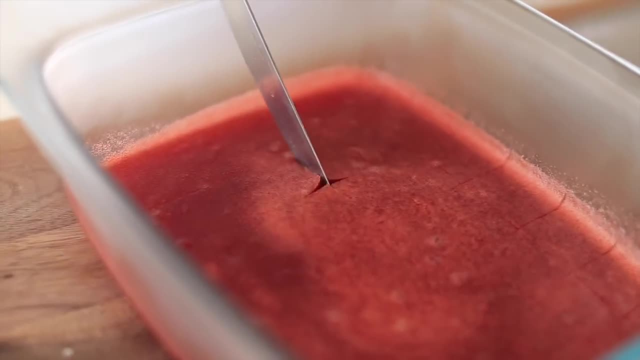 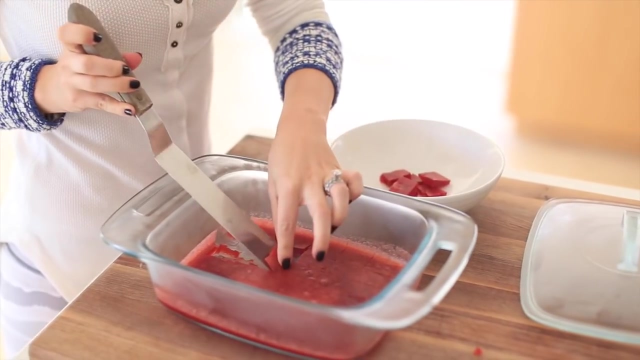 You can kind of do whatever you want with them. But again, with this recipe, very similar to the fruit roll-up recipe, I probably would have preferred if I strained the seeds and didn't have the seeds in there. But I will say they tasted really tangy.